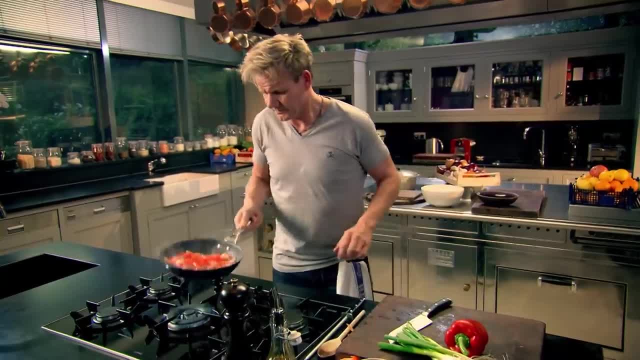 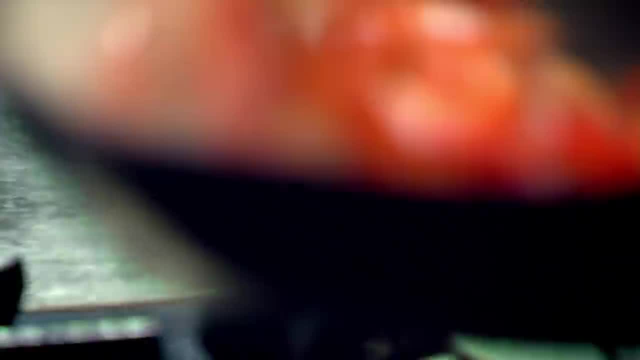 Roughly. chop a red pepper and add it to the pan. The peppers and the bacon take the longest, so they've got all day. You've always got to go in first. Now sauté them off. The peppers have been cooked now. 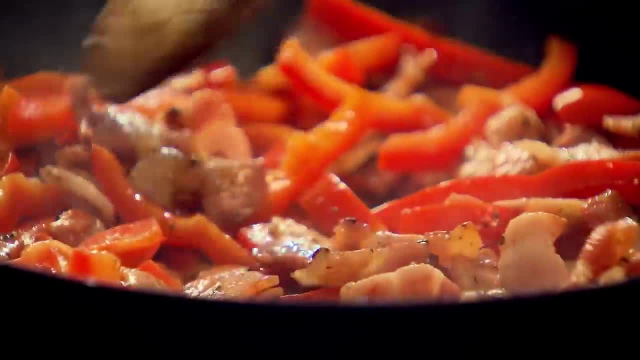 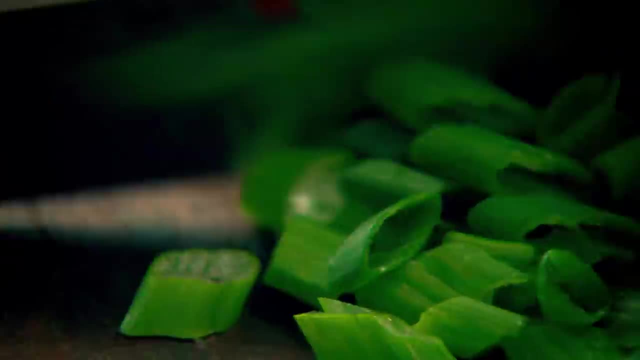 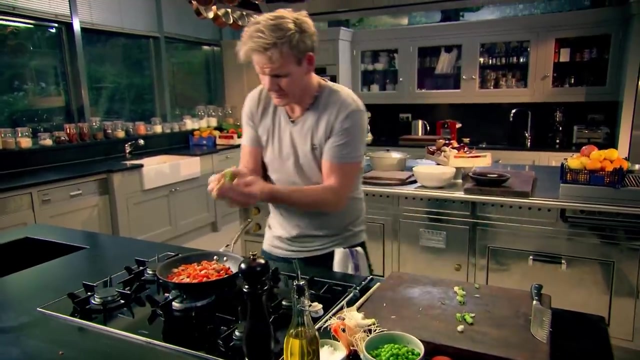 from that sort of rendered fat from the bacon, And then the spring onions. Just bunch them up and slice them. I want them on an angle so they come like little green diamonds. Spring onions in. Now for the eggs. Crack in the eggs. 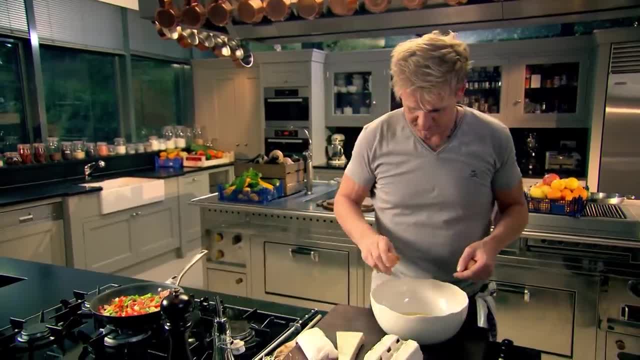 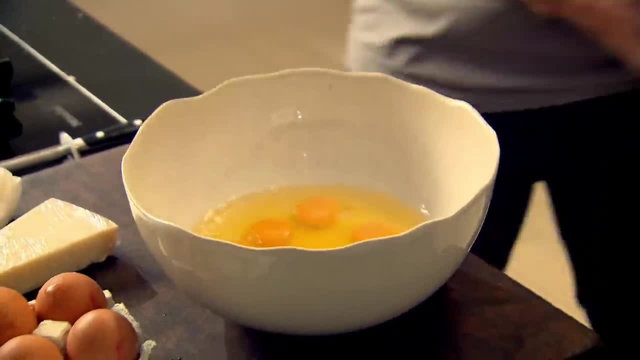 For that size pan, seven or eight eggs. I want to fill it right to the very top And, more importantly, when I turn this out I want it like a gateau, Nice and thick, so we can slice through and see all those wonderful veg. 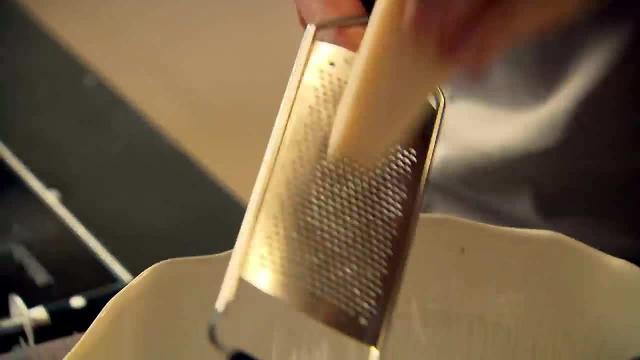 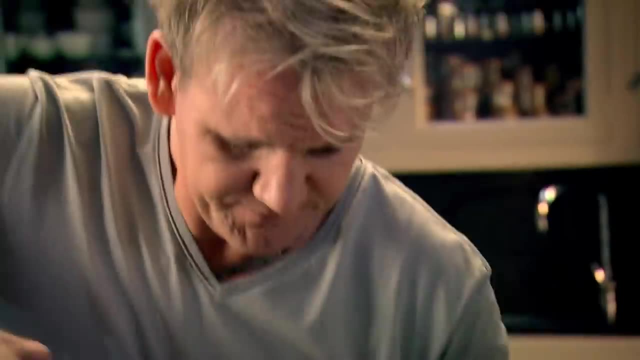 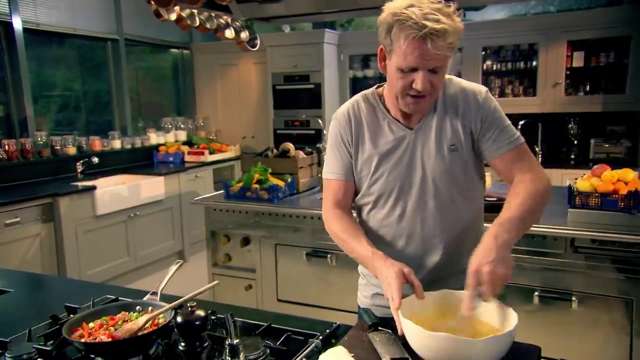 I'm going to season the eggs with some Parmesan cheese- Be quite generous- because it adds a really nice saltiness. I'm going to add a little bit of pepper, Fresh ground pepper, And then whisk, Whisk up those eggs nicely. 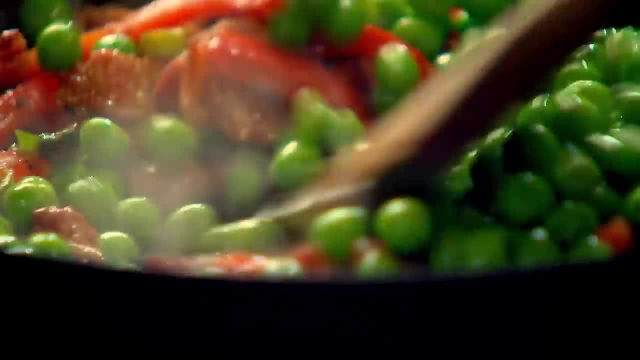 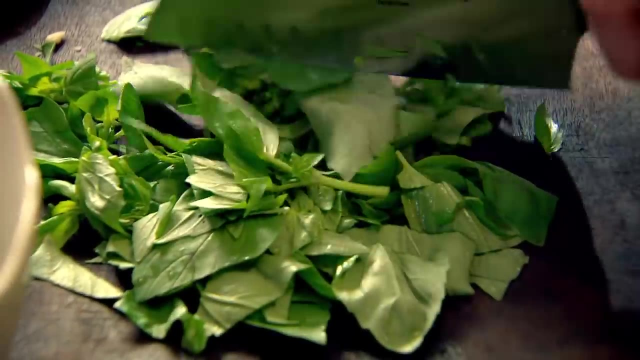 Then add peas to the pan And, to give the dish a wonderful aromatic freshness, some fragrant chopped basil. I want to chop that sort of roughly because I want to see those flecks of green going in. I want it looking charming. 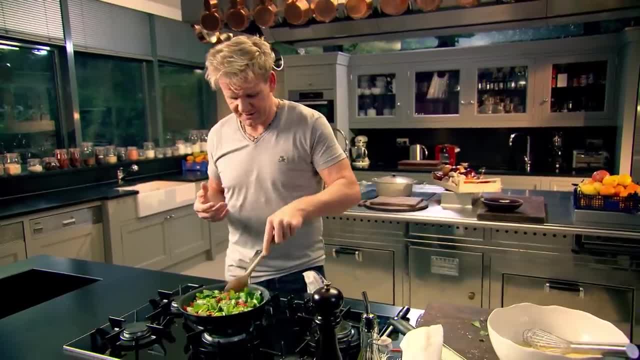 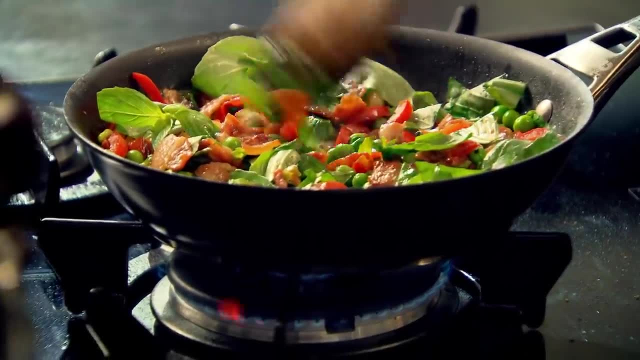 And how many times have you seen a, a dull omelette Frittatas, in my mind, really helped encapsulate the magic of having savoury eggs cooked beautifully but with texture. Now, just before we add the eggs, 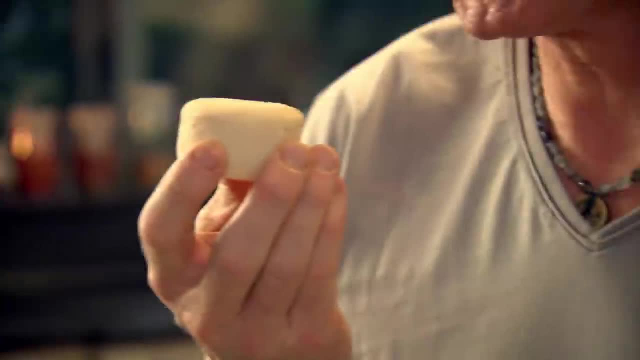 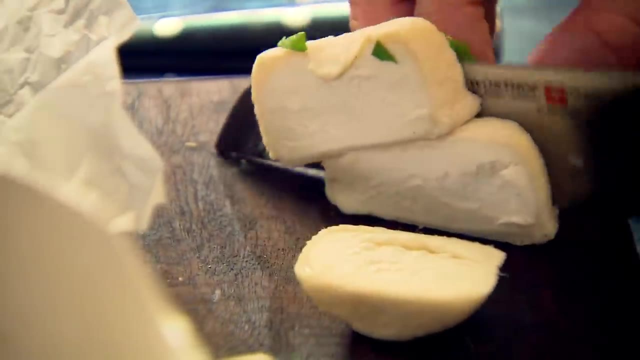 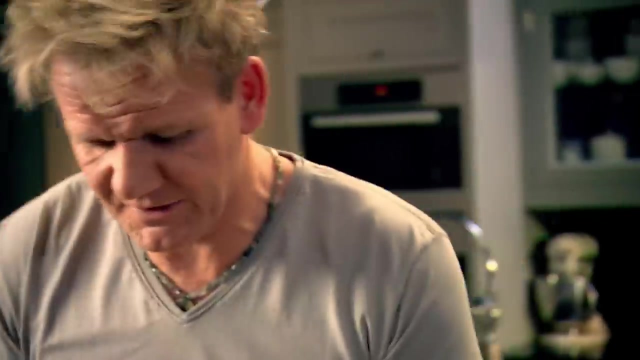 I've got this beautiful little goat's cheese and it's strong and powerful, So I want to slice it into little chunks And then just have it dotted around. I want to discover these little pockets of creamy goat's cheese. Now slowly add the eggs. 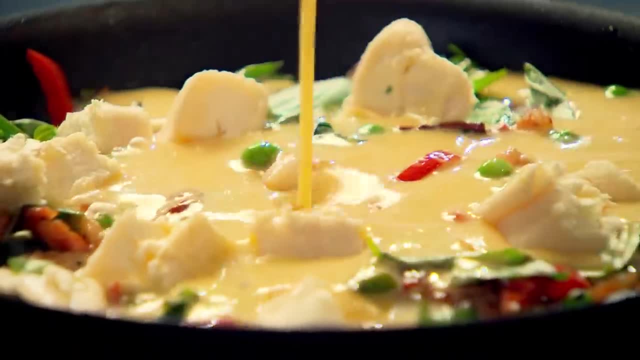 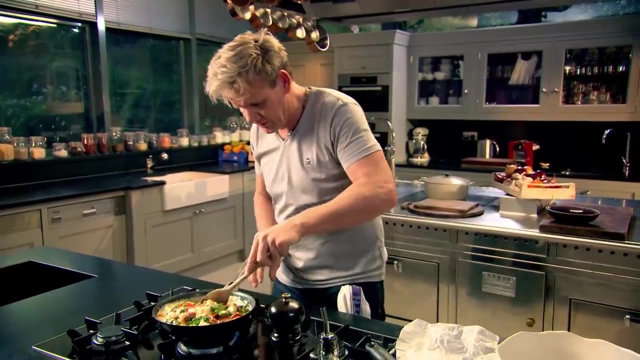 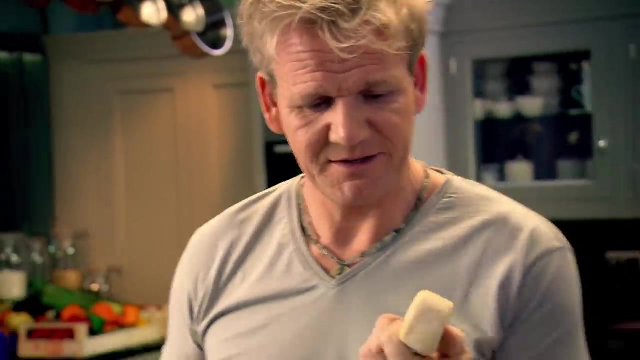 Fill that right up And get your spoon. Now just let all that egg go down to the bottom, Bring it back up to the boil And sort of clean round the sides, And then some of this delicious salty, creamy goat's cheese over the top. 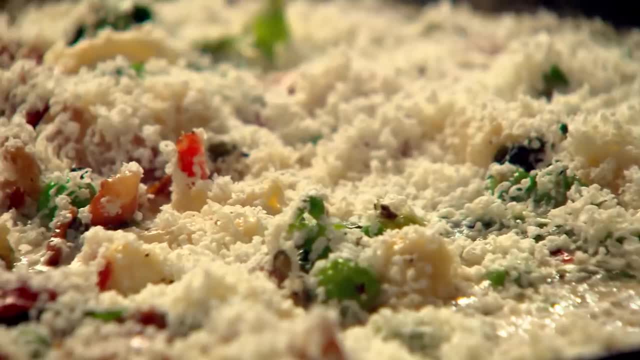 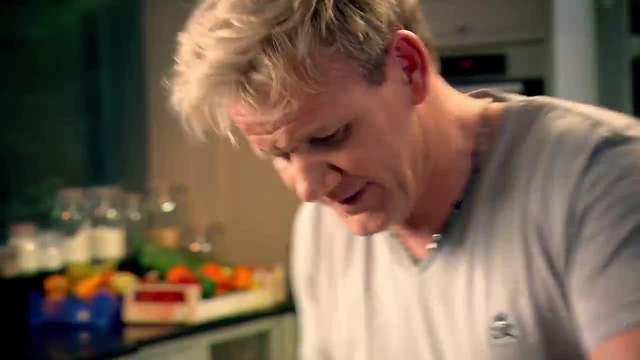 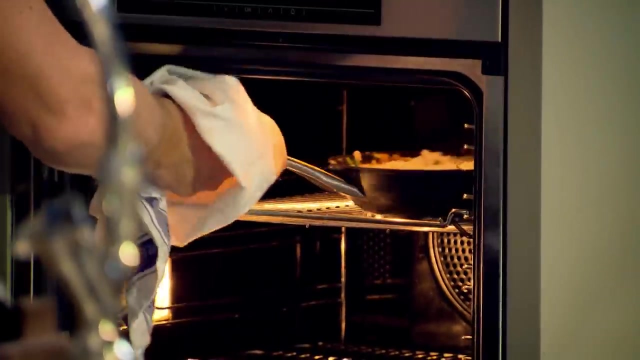 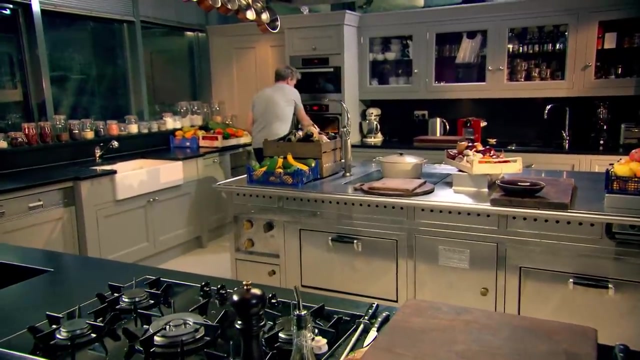 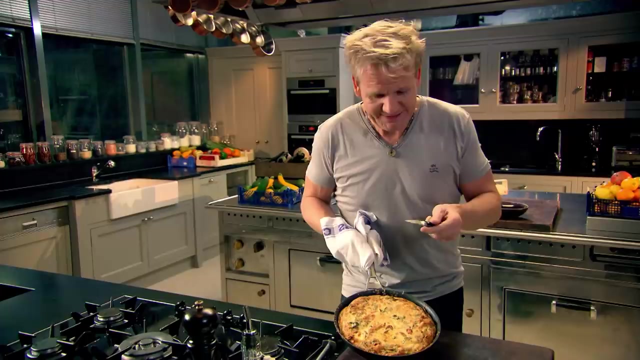 Now I want it melting like a a perfect slice of cheese on toast. Nice, Now, from there, turn the grill on for four to five minutes. Mmm Now, just looking at that delicious. Take a little paring knife. 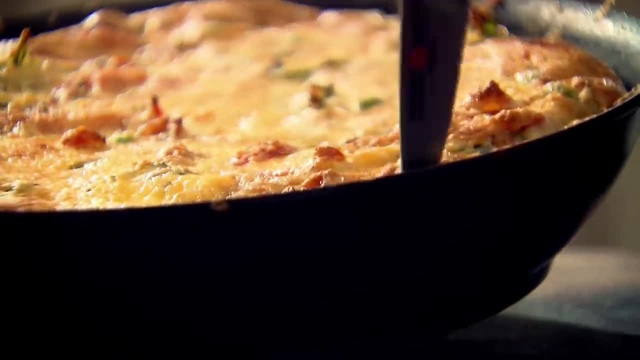 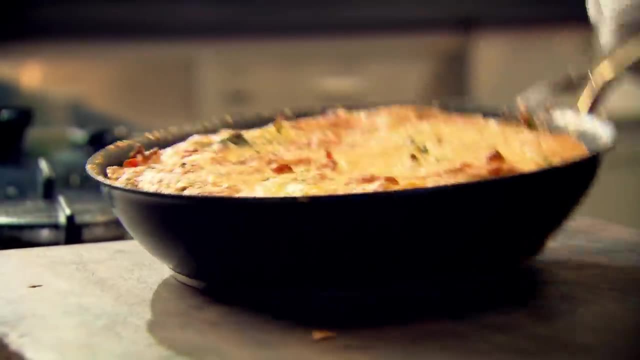 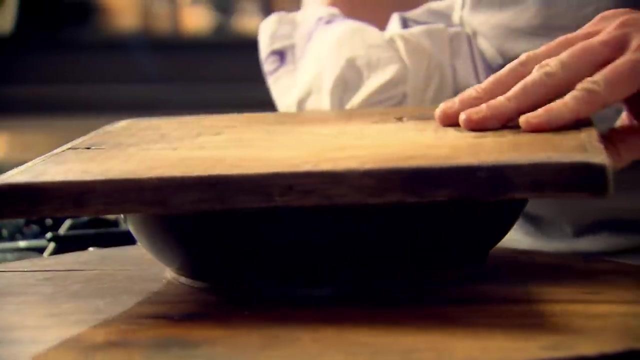 and just make sure it's released on the sides. Just take your pan and tap. That will hopefully release the tartar from the bottom of the pan. Now put the board over the pan, Turn that gently And just shake. 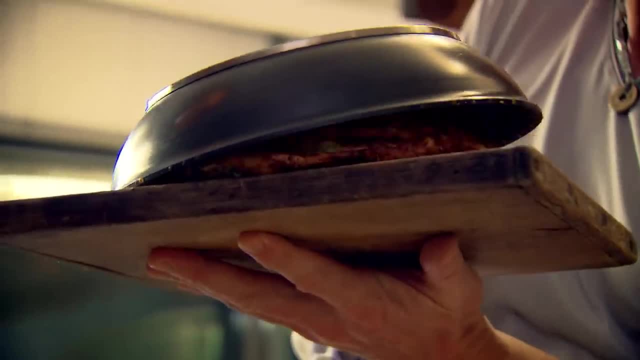 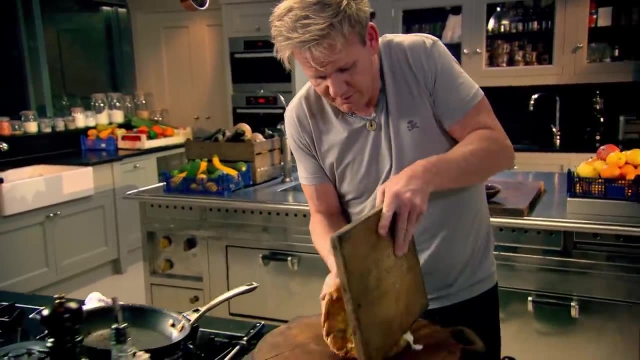 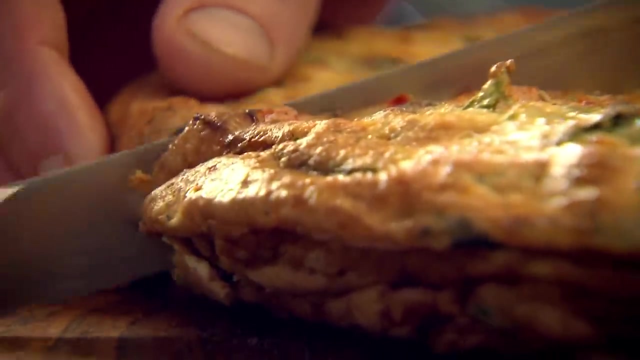 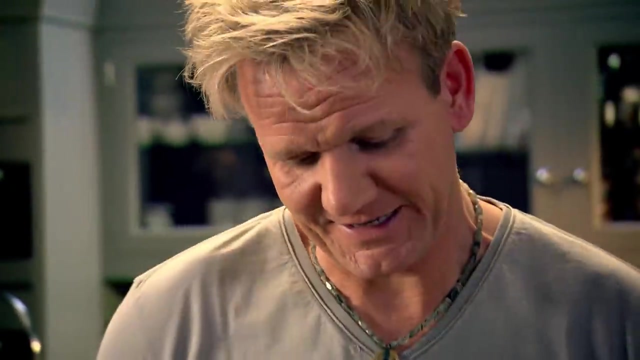 Say a little prayer And lift off the pan. Beautiful Now from there on. There it's there. look Now, slice through Mmm. You can see how soft and creamy that is in the centre And that goat's cheese is just melting. 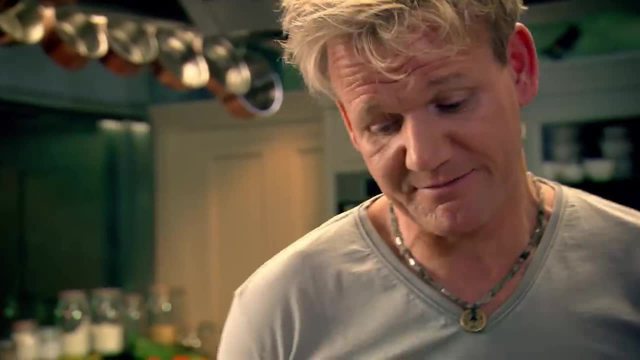 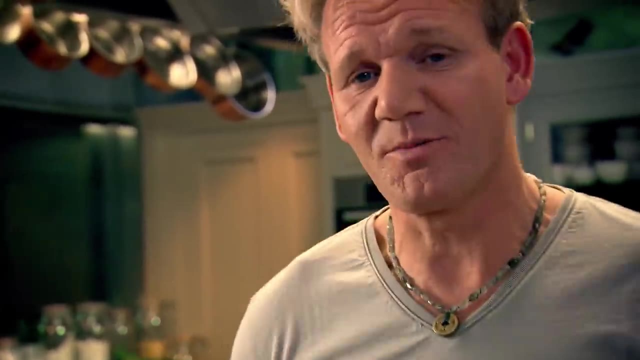 almost like a little sauce inside. So exciting, But more importantly, it's so easy to do. It's got texture, It's got creaminess, And that, for me, will beat any omelette for brunch, Served with a stack of hot buttered toast. 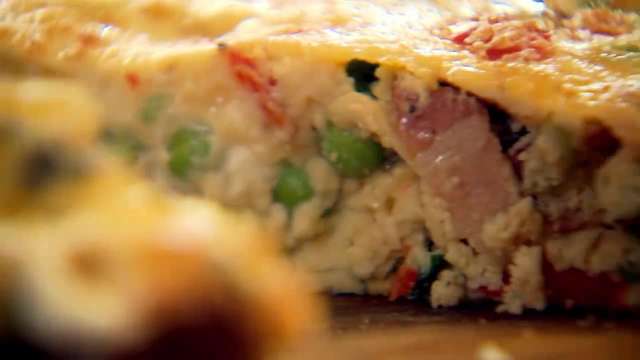 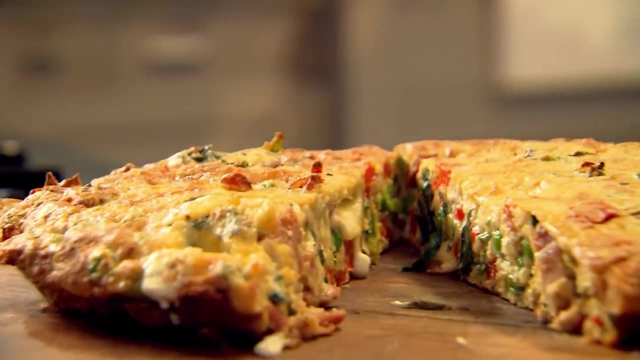 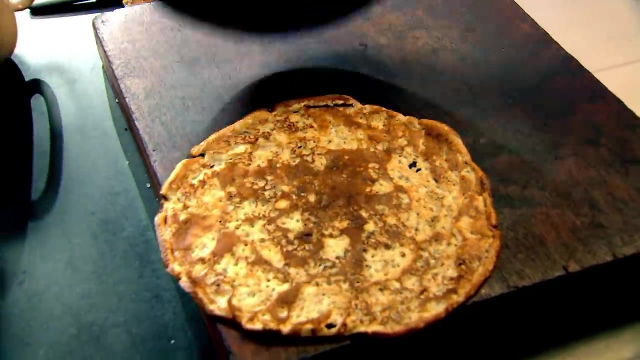 and a steaming pot of coffee. this easy frittata turns the humble egg into the perfect dish for kicking off the weekend. Brunch should be a laid-back affair and a treat, So the dishes need to be easy to cook but never boring. 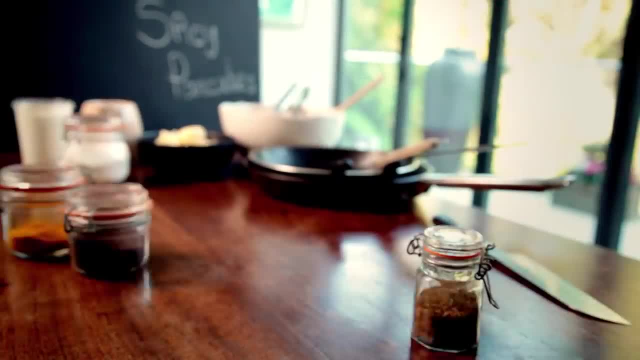 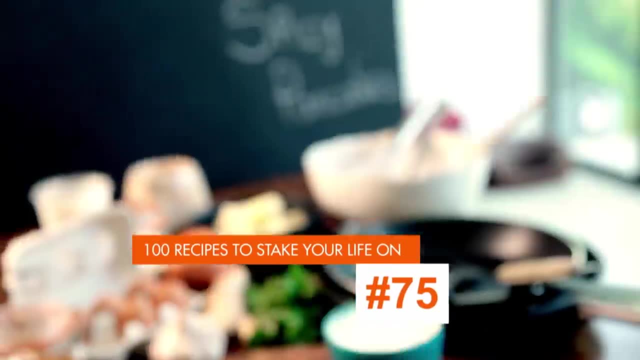 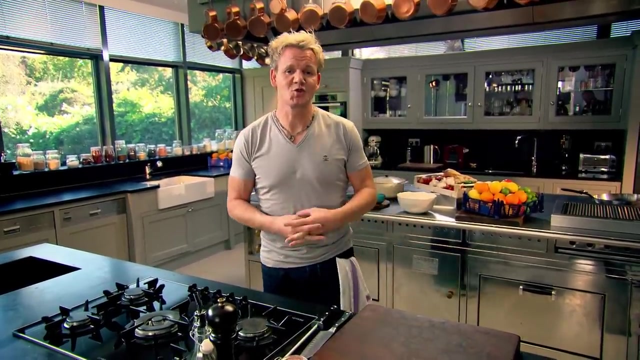 My next recipe takes the humble pancake to a whole new level of flavour and excitement: Soft, fiery and irresistible Spicy pancakes. One of the secrets to good cooking is learning to use your imagination. When it comes to brunches, you don't have to stick to the old standbys. 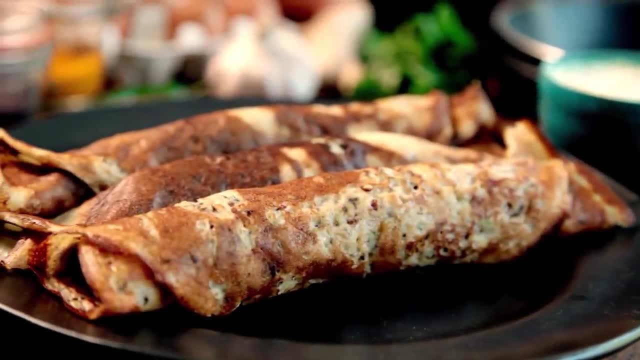 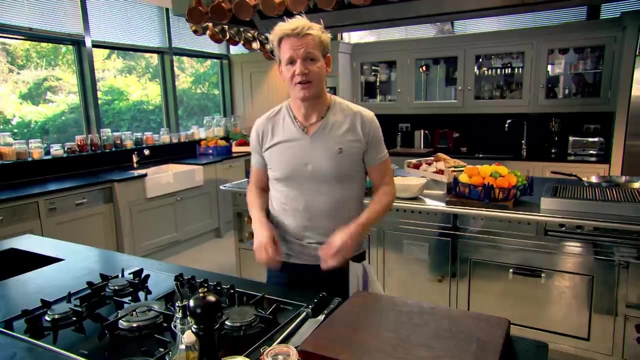 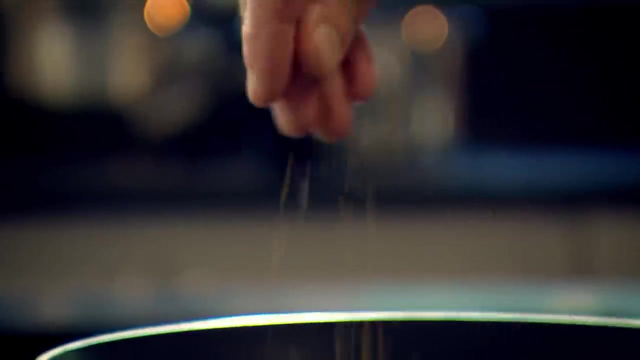 These delicious spicy pancakes are a really great alternative but, more importantly, so easy to do. Start off by toasting your cumin. It's a dry roast, basically Non-stick pan, Just a touch of seasoning. The salt helps to dry out the cumin even more. 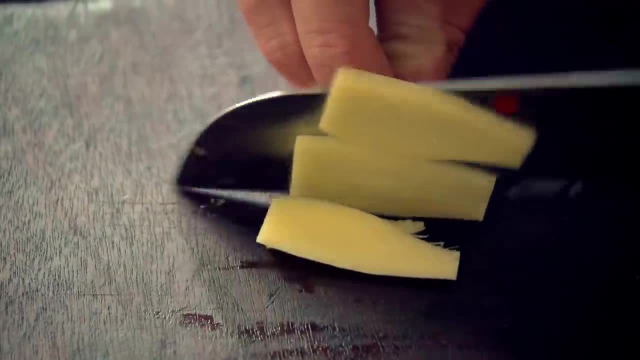 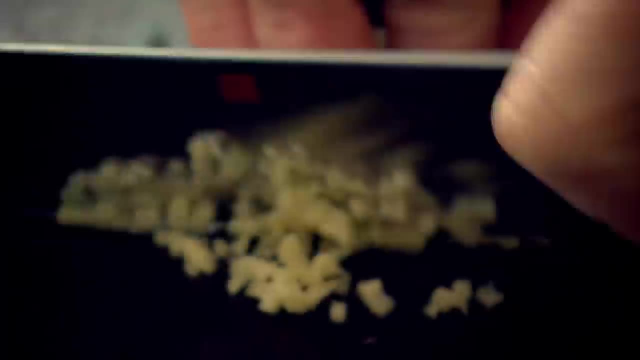 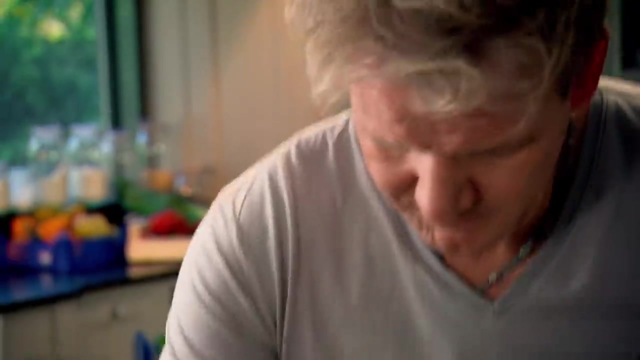 And then fresh ginger, Slice them nice and thinly, Stack it back up And then just slice Nice little thin slices in there And then keep that bunched up. Shape the chilli Just like this. Removing the seeds will prevent things getting too hot. 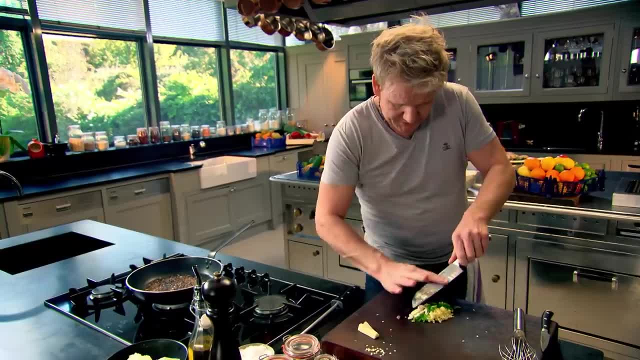 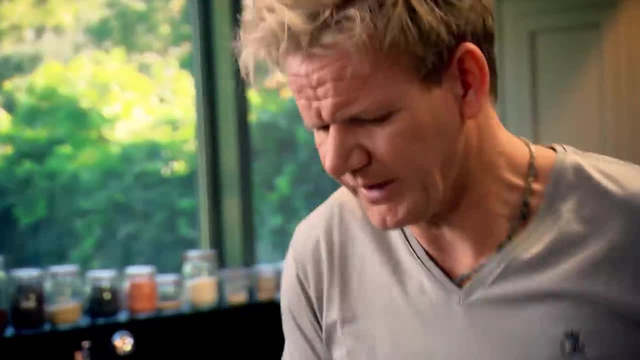 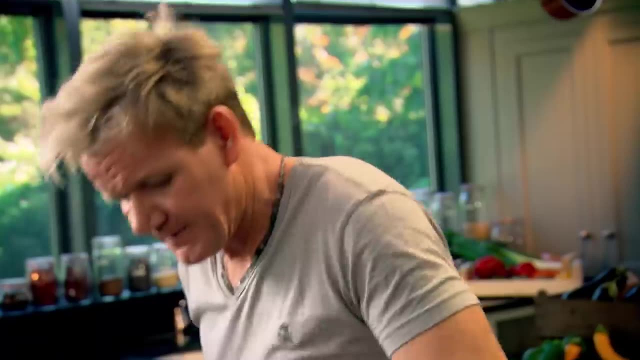 Now garlic: Nice, Now add olive oil to your toasted cumin seeds and in with the garlic, ginger and chilli. Lovely, And it feels strange when you talk about garlic for breakfast, but the time I spent in India, everybody was eating something savoury for breakfast. 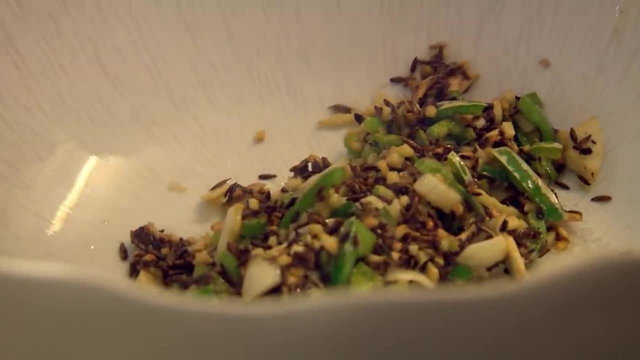 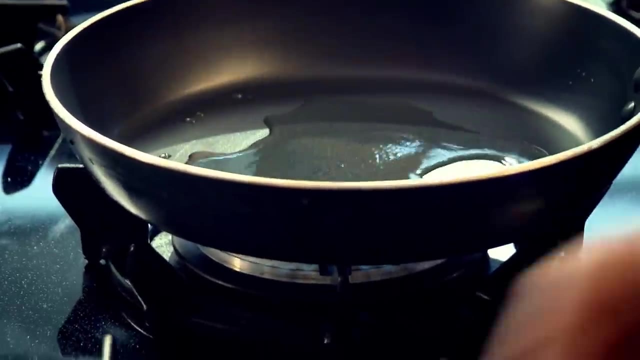 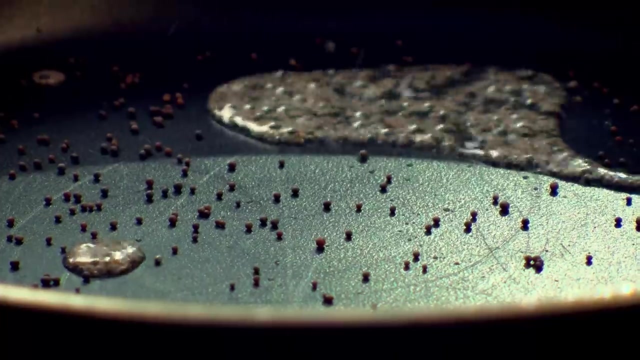 It was extraordinary- Into your bowl And set aside. Next the pancake filling. Add olive oil to a hot pan. Mustard seeds in. Now they'll start dancing the minute they hit the pan, Mmm. Then finely slice an onion. 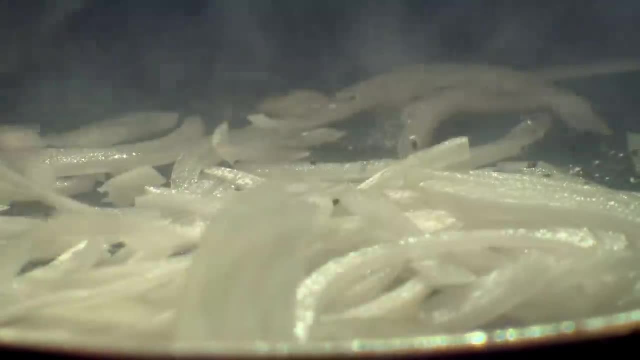 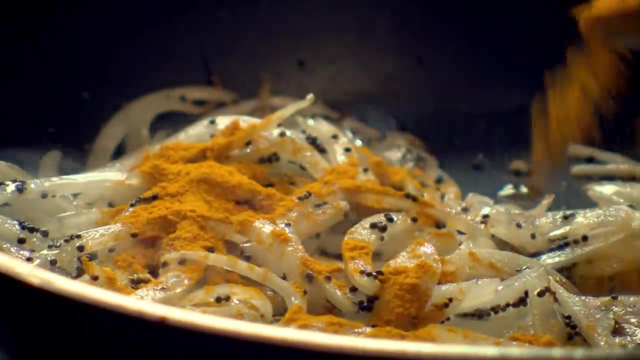 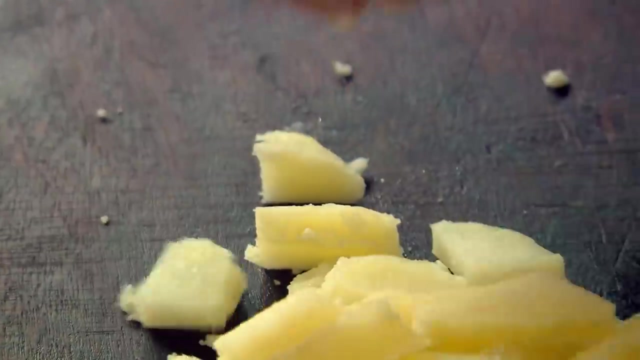 Onions in A little teaspoon of turmeric. Sprinkle that in And look at the colour. An instant change. Leftover potatoes: Just slice them. The smell is incredible. Potatoes in now. Spread the potatoes across the pan. 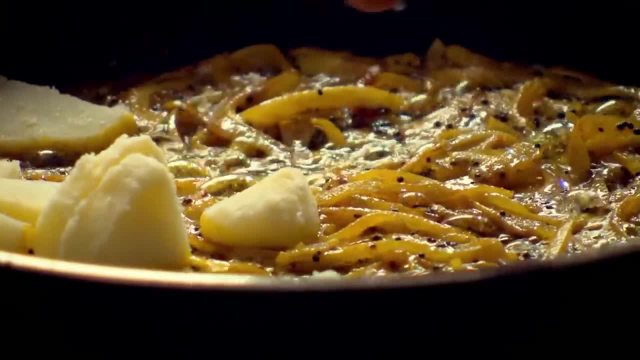 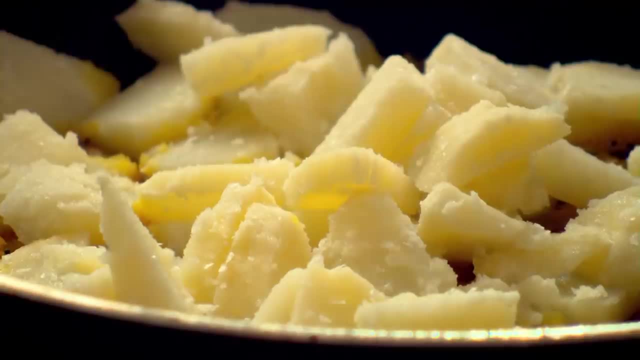 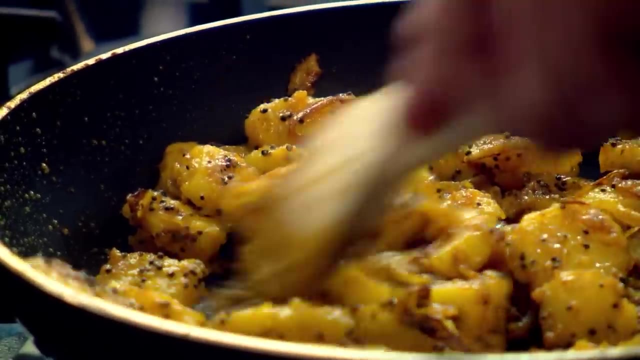 While the potatoes stain, I want them sort of absorbing all that really nice turmeric. Actually, like a sponge, Season those potatoes and it really helps to bring out the spice beautifully. They're ready, Turn off the gas and let them sit there and absorb all those flavours. 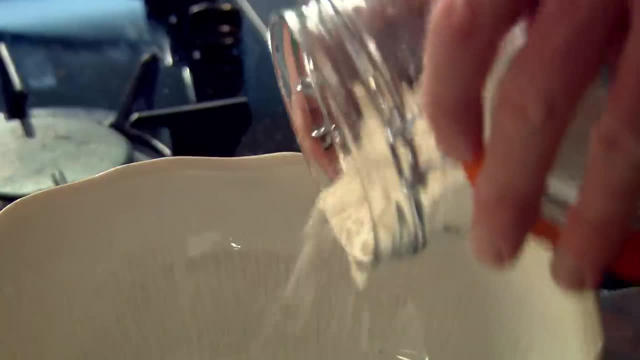 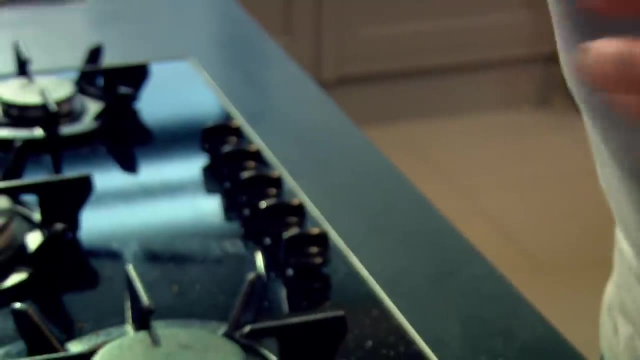 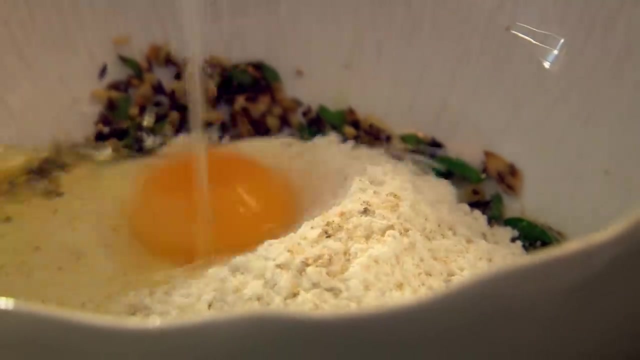 Back to the pancake batter. Add plain flour to your cooled garlic, chilli, ginger and cumin seeds. A touch of salt and pepper. Nothing worse than a bland pancake. One whole egg Milk. Hold the jug with one hand and whisk together. The secret is to get that really nice, smooth paste. 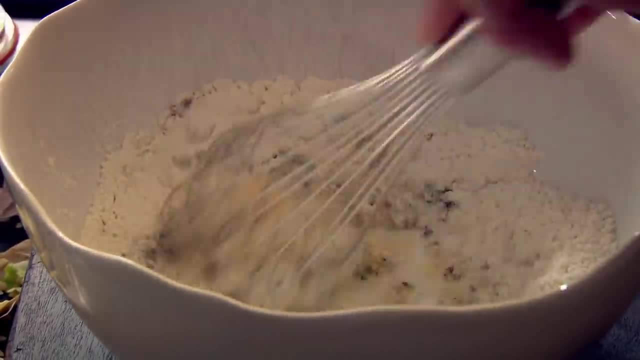 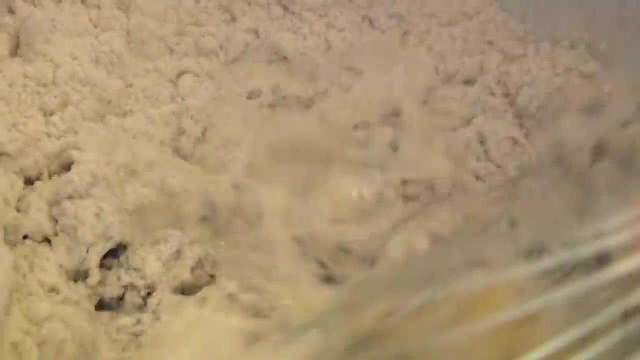 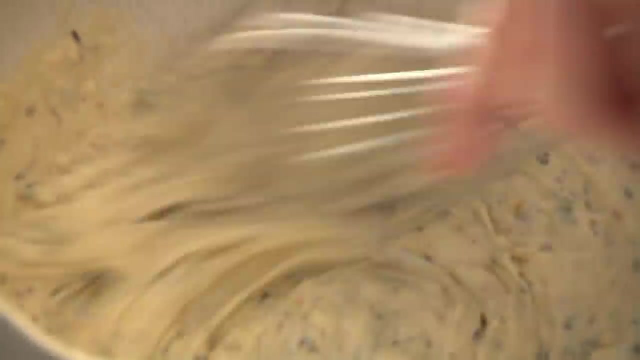 But whisking that egg first brings it together And then you're milking. Don't put all the milk in, Because then you're going to get a lumpy pancake mix And if you put less milk in, It really helps it not go lumpy. Look at that. 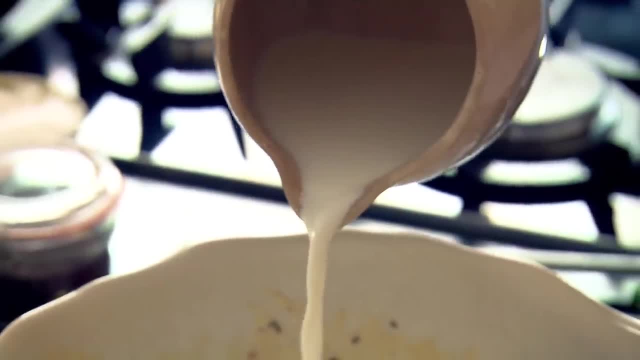 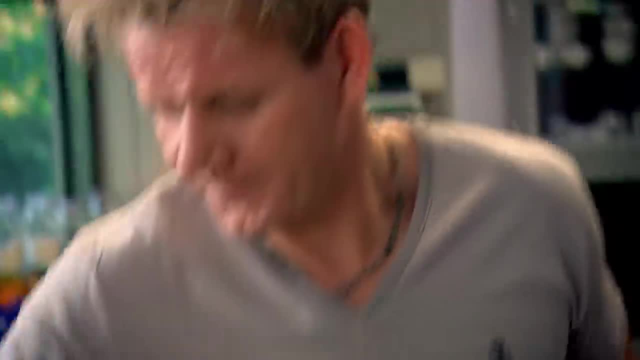 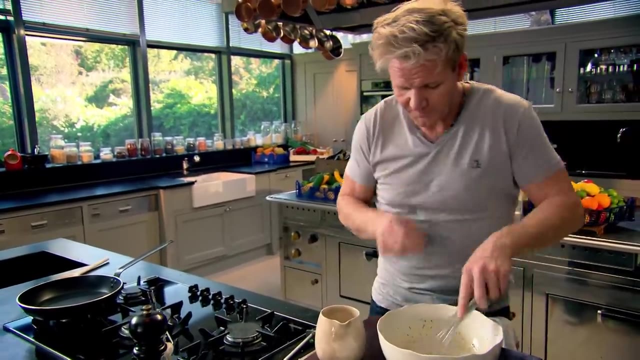 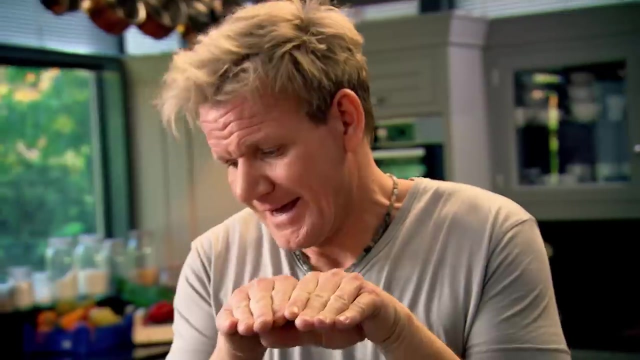 Milk in. The secret for me is to have a nice thin mix. Now just a little teaspoon of oil. That helps to bring a nice crispy edge to the mixture. Now just a taste. That's the texture Pan on. The larger the pan, the better It helps to create that nice, thin, even surface. 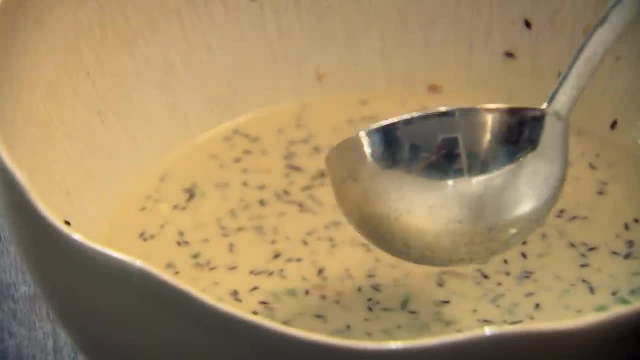 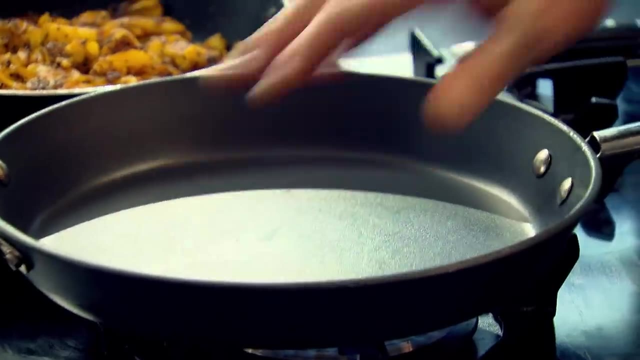 I want that mix going all the way around the pan. Before you put the mixture into the pan, Make sure you give your pancake mix a really nice stir Pan. it's nice and hot. Turn down the gas, A touch of olive oil in, Get that nice. 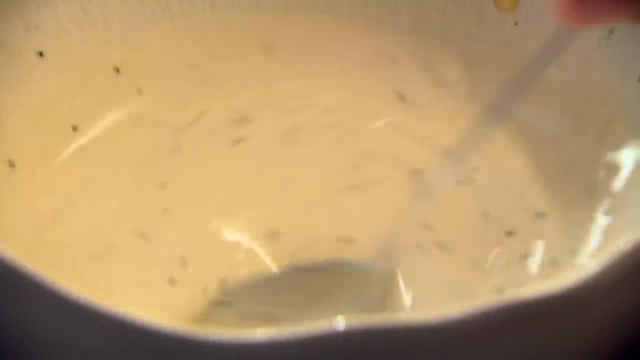 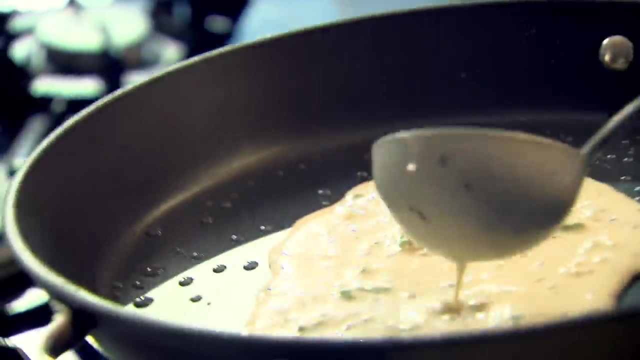 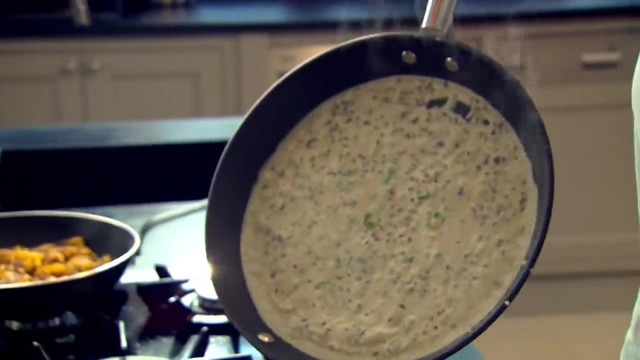 Whisk with one hand Pan to the mix In One and a half ladles And then roll it around. It goes really nice and thin. I want to see the ginger, the garlic. That's what I'm looking for In there. Now back onto the heat. It only starts to remove. 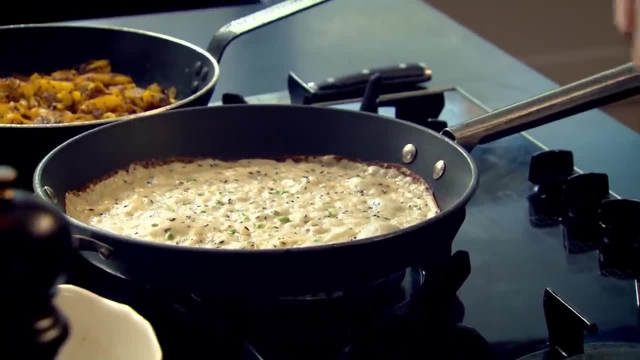 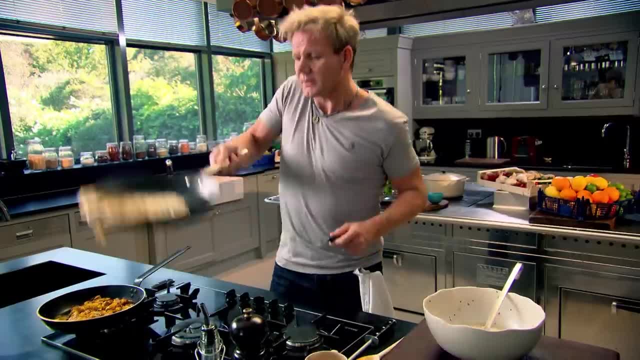 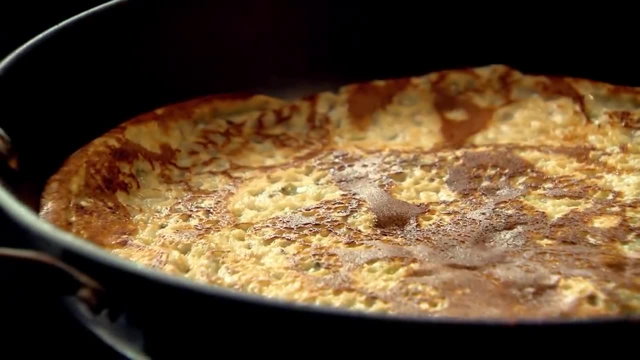 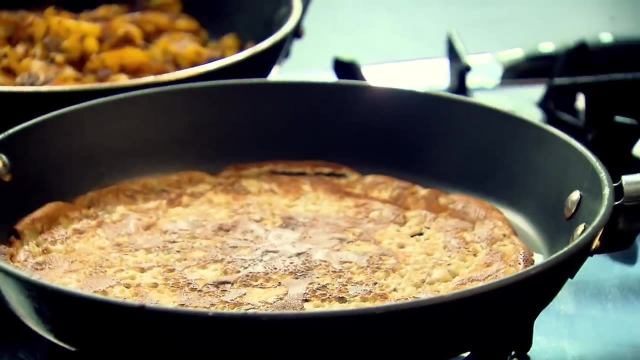 That releases it And then just shake it to the end And toss. If you haven't got the confidence of tossing, Then use a spatula and turn it over. Now, that's exactly what I want: That nice sort of crisp edge around the side. The colour on the pancake is so important. 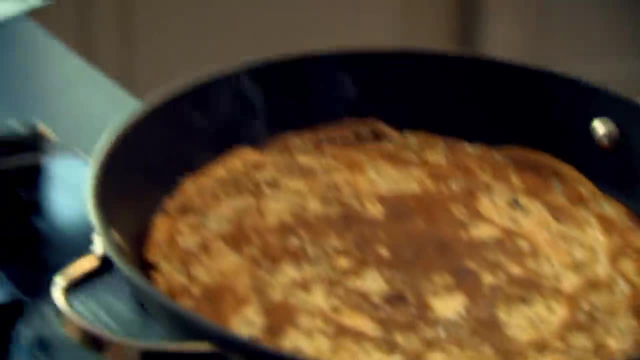 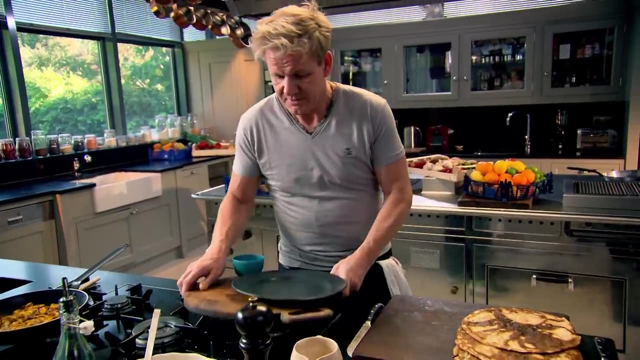 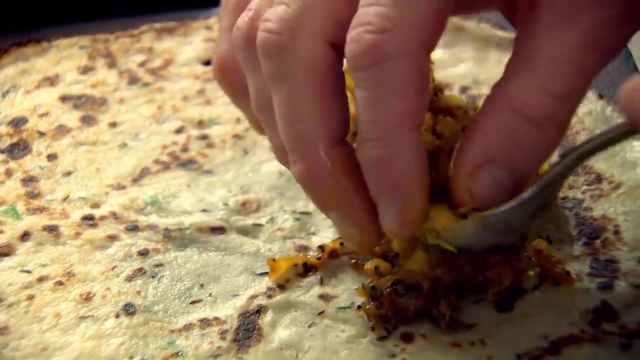 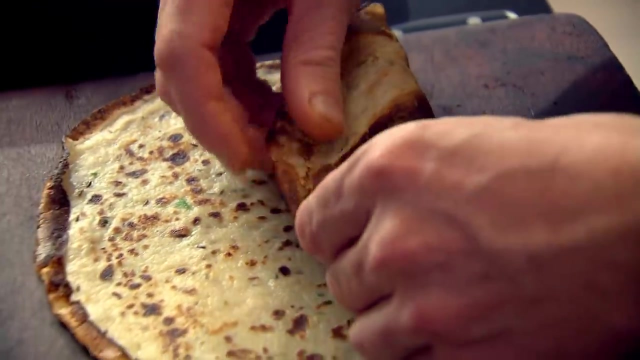 Now roll it round And just let it slide out Beautifully. Mmm, Now for the exciting part: Filling them. Take your potatoes, Just sort of have a really nice imaginary line And then just very carefully roll that Nice and tightly Tuck it underneath there. 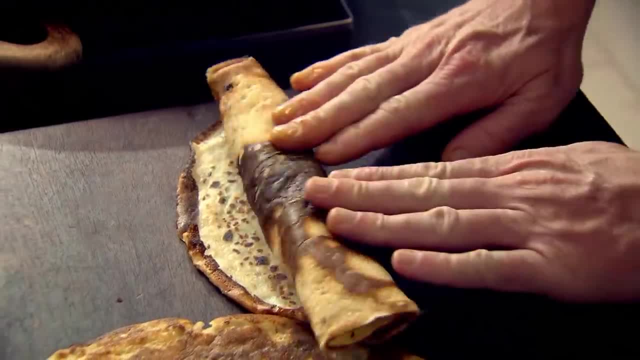 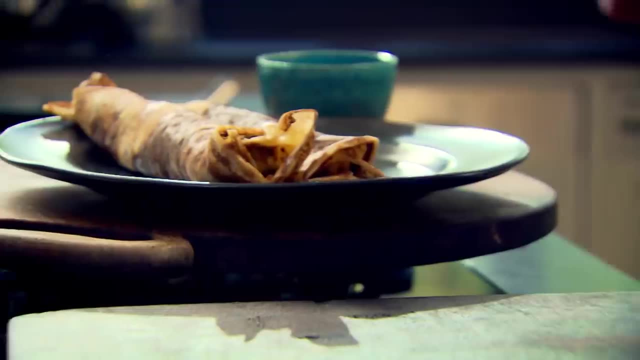 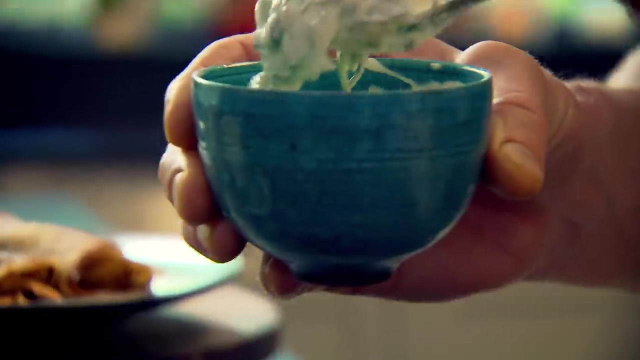 Pull it back and roll. There we go. Beautiful, The delicious pancakes are ready to eat. But with a simple dipping sauce They'll be a real treat. Just mix chopped coriander with natural yogurt. That's really nice Cooling agent. Sit that on the side And that, for me, is a great brunch. 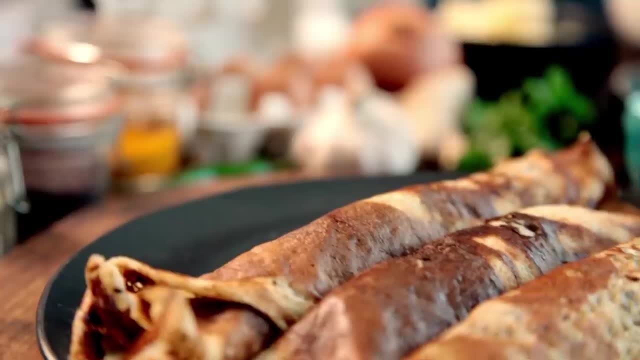 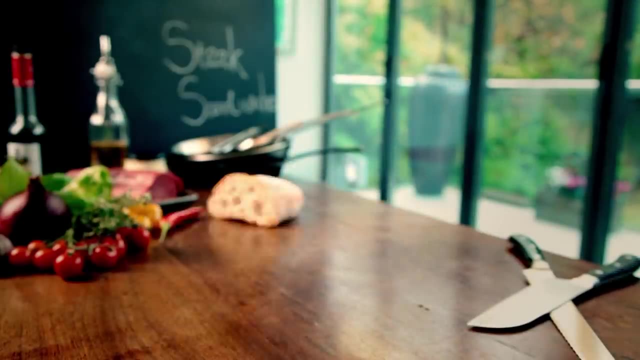 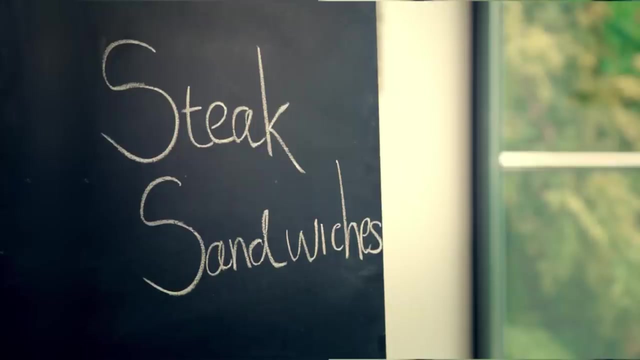 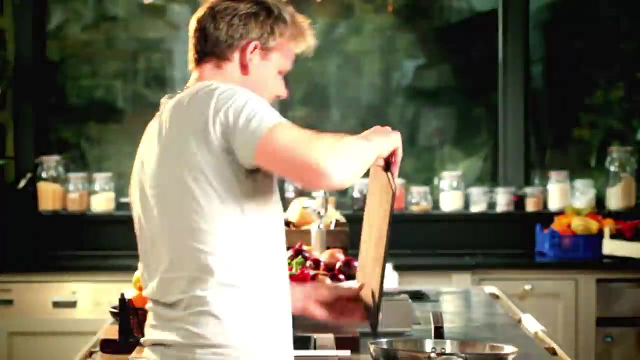 Delicious spicy pancakes, Amazing And one of my all-time favourites. A dish that always comes with a meal, creates a stir- is the daddy of all brunches: steak sandwiches. For me, the secret of a great brunch is fun and casual, fuss-free cooking and everyone helping themselves. 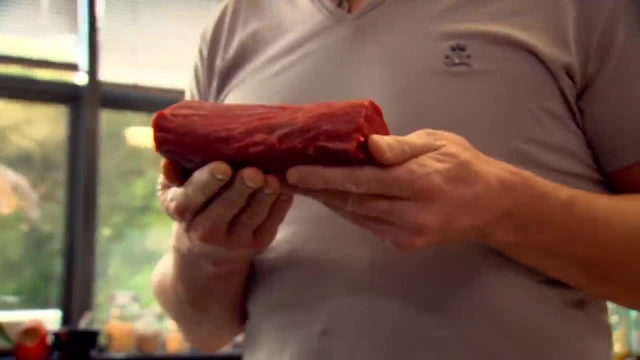 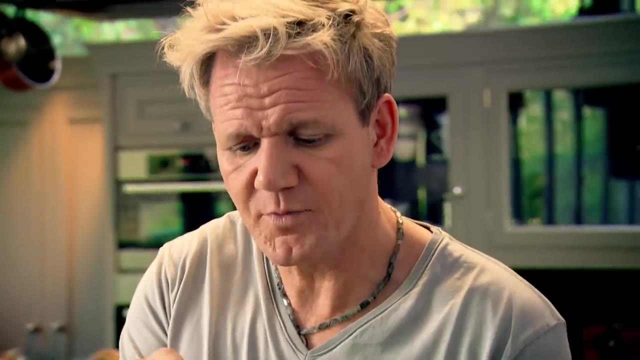 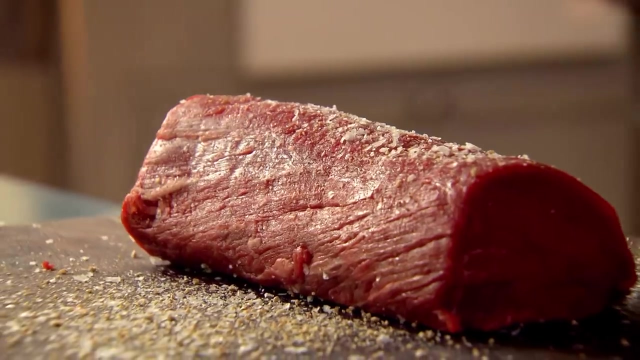 This is the ultimate steak sandwich. You want the Rolls Royce of beef. It has to be fillet Now season it beautifully. I like to open up the top of the pepper mill to increase the size of the pepper in the steak so it gives that bit of heat. 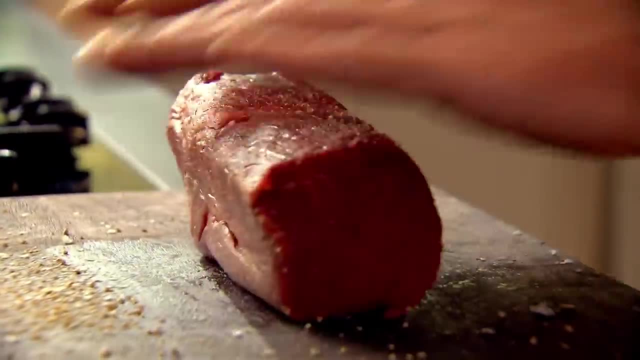 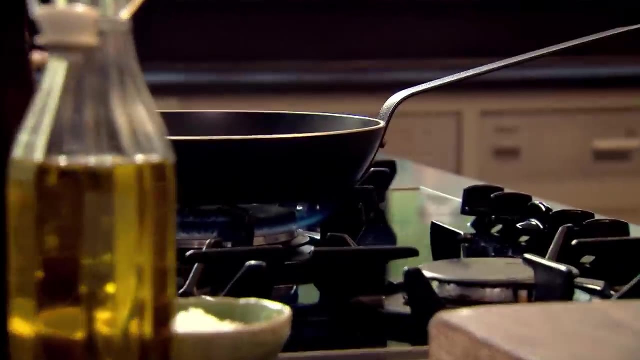 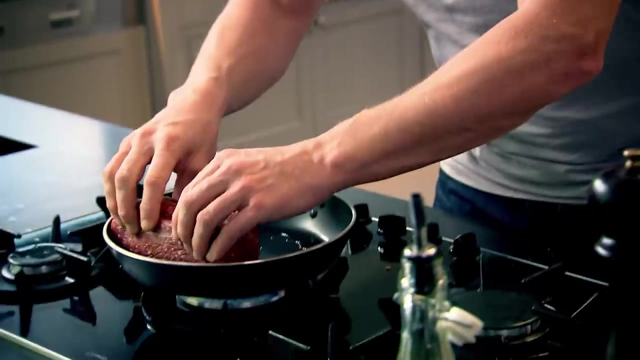 Nice little chunks You just roll now nicely all the way around. Now slice the garlic in half, Pan nice and hot Olive oil in, Hold the steak and just place it into the pan. Don't drop it At the front of the pan. 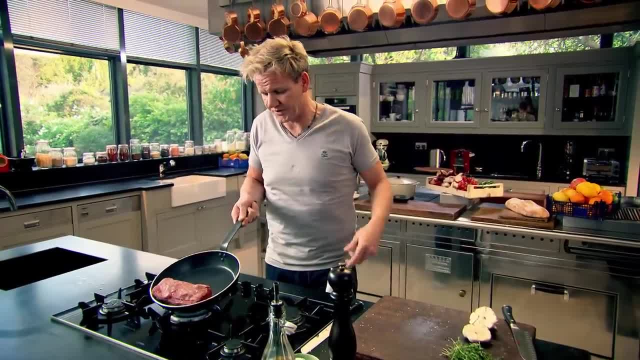 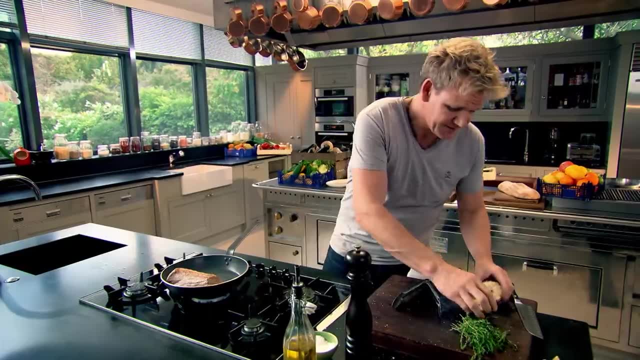 I'm going to tilt the pan forward to cook the back of the steak. dual purpose: Now roll it back and sear it underneath. Next, my garlic And roast that garlic. Thyme, fry that thyme. I want to hear it. 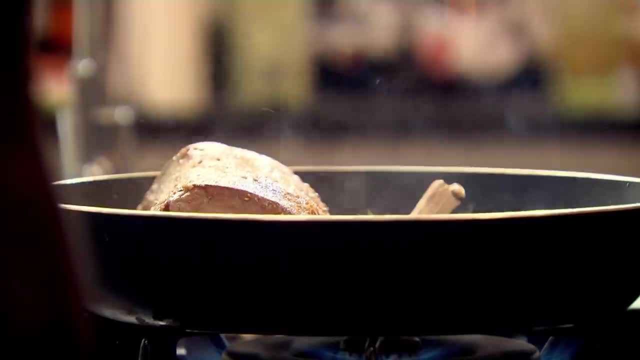 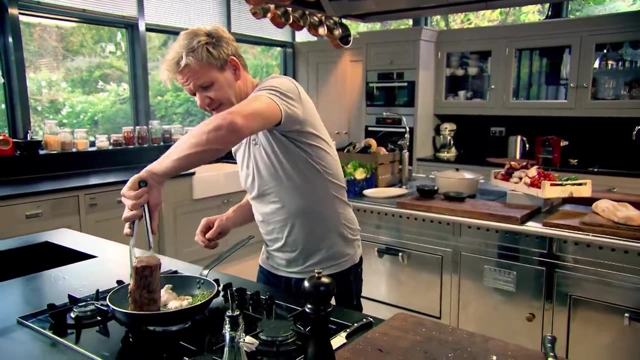 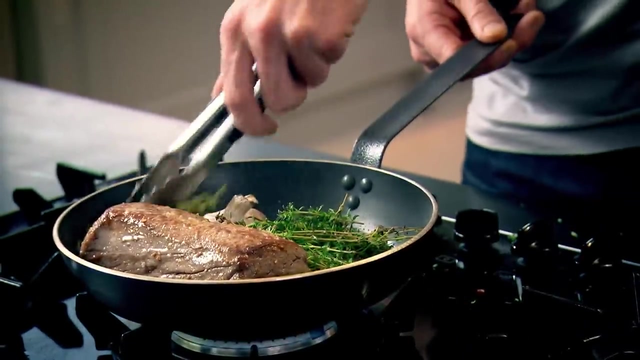 We're not looking for a lot of color because you're going to dry out the fillet. So just one end, turn it back down and sear the other end in. Lift up your thyme, place it on top of the garlic. 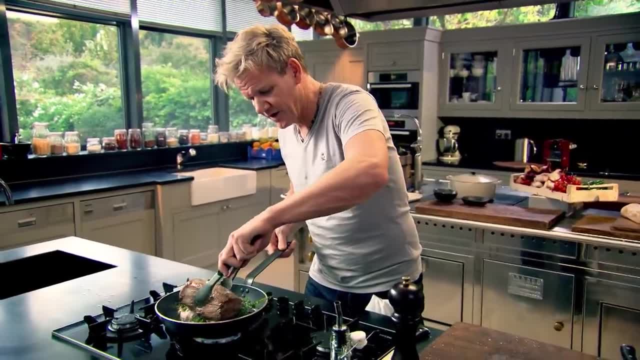 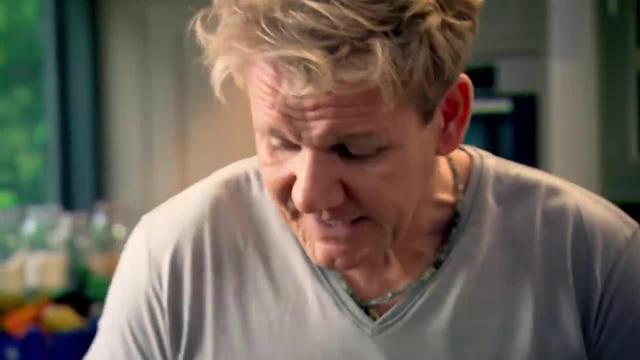 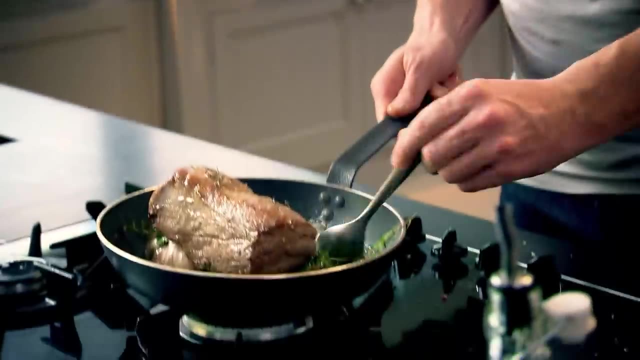 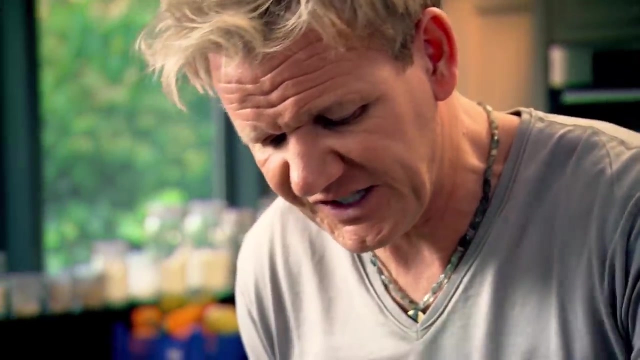 There. Lift up your fillet and sit that on top of your garlic Butter in. Take a spoon, tilt the pan gently, lift up and baste. I've got that scented garlic thyme flavor. The steak's going to cook evenly because it's sat on a little. 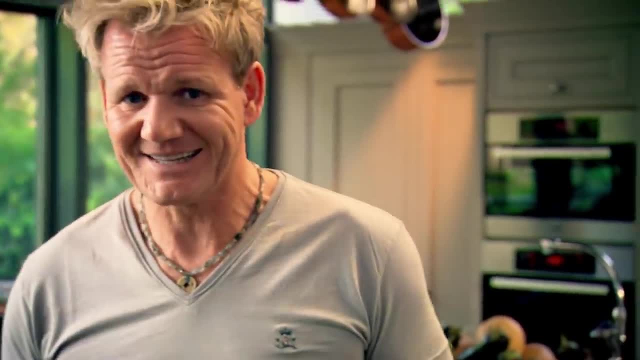 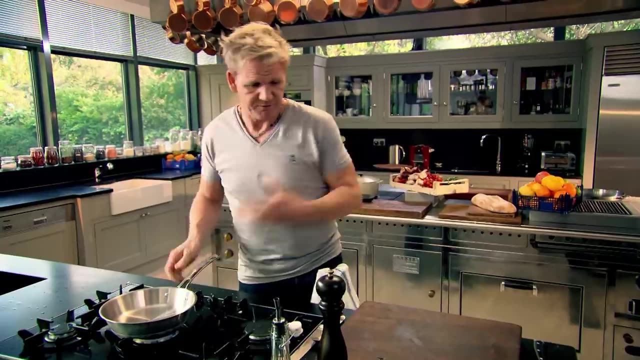 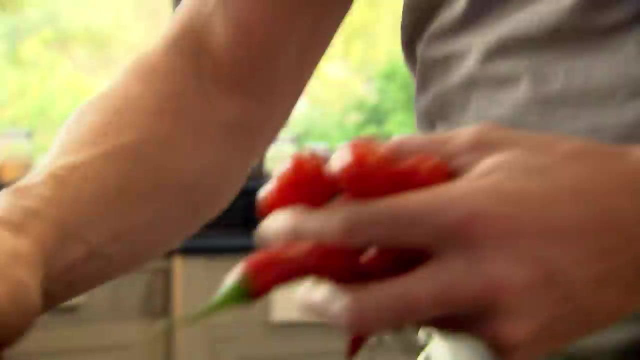 a little bed in the oven for eight to ten minutes. Pan on For the relish. you think of a steak sandwich. you think of a sort of nice heated tomato relish. To make the relish finely dice a red onion. 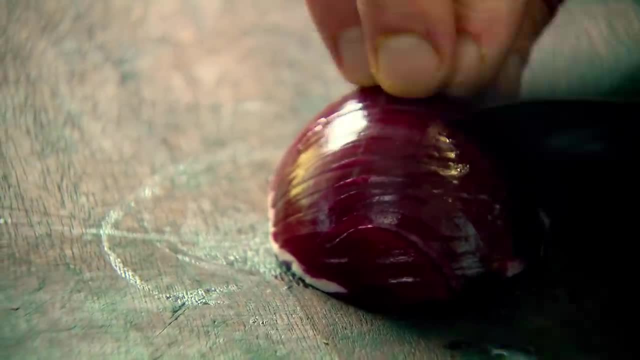 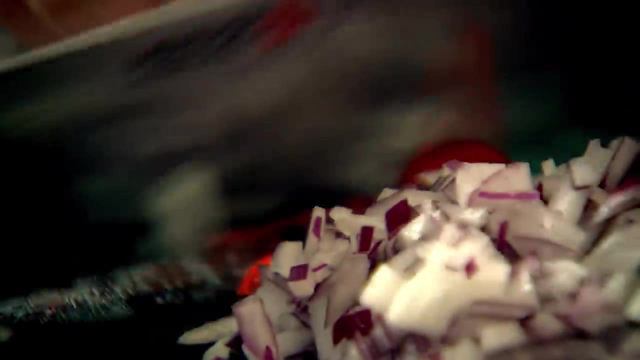 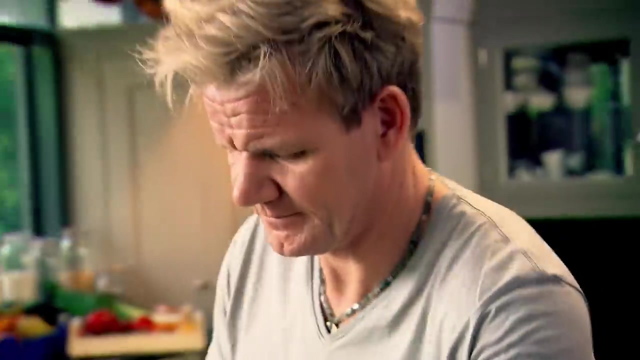 Three-finger rule: One in front, two behind, Through and chop, Wow, Next relish, Next relish. Roughly chop a chili, keeping the seeds in for extra heat. Start off with the olive oil Into a pan. 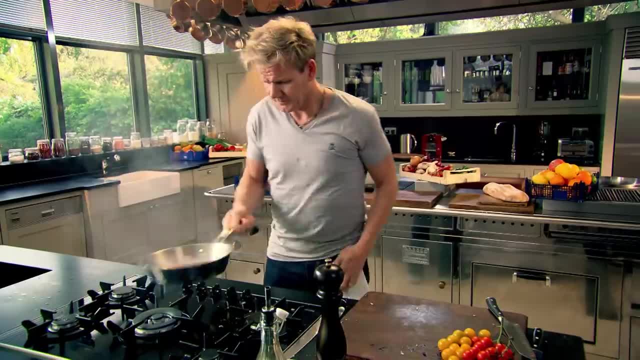 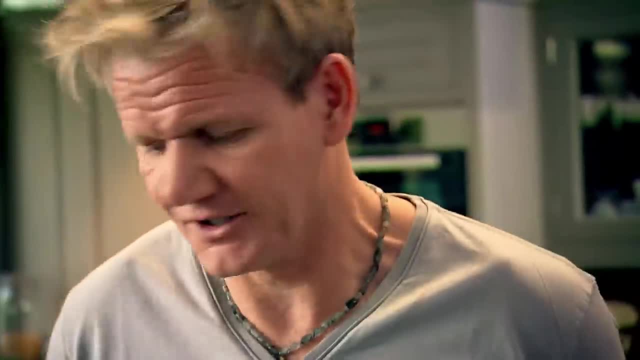 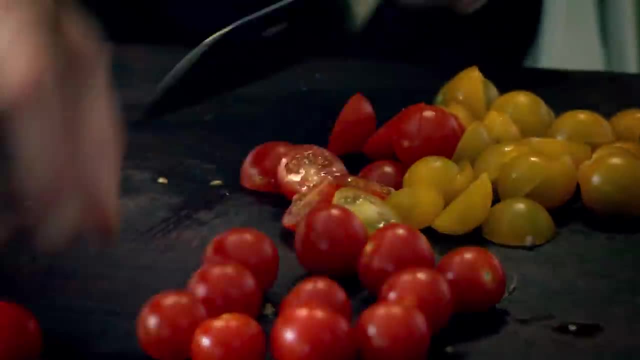 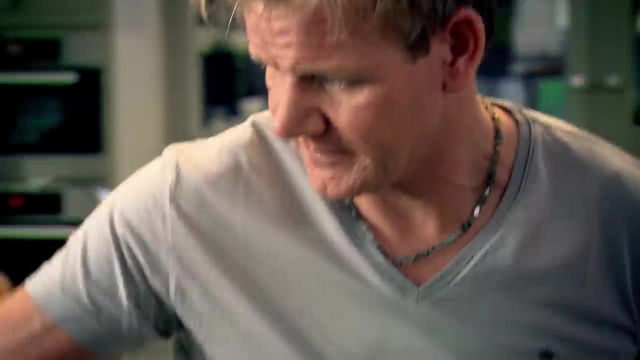 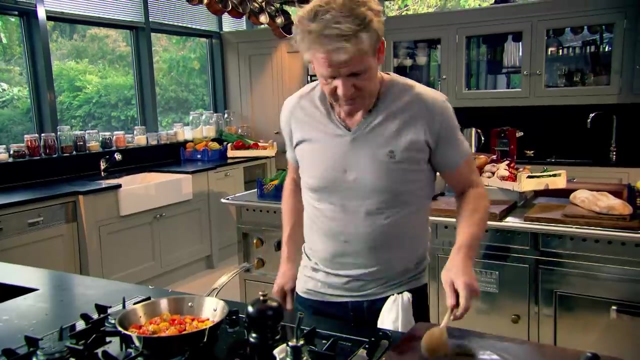 Onions, chilies Generous with the olive oil. I want a nice sort of rich, silky relish From there. take your tomatoes. You can just use red tomatoes, but these yellow and red make the perfect combination. Now put your salt in pepper and then roast those tomatoes off. 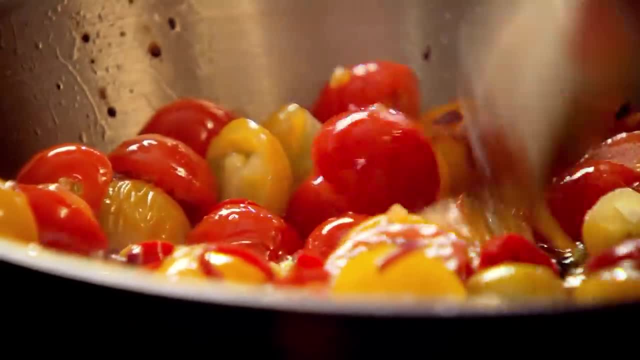 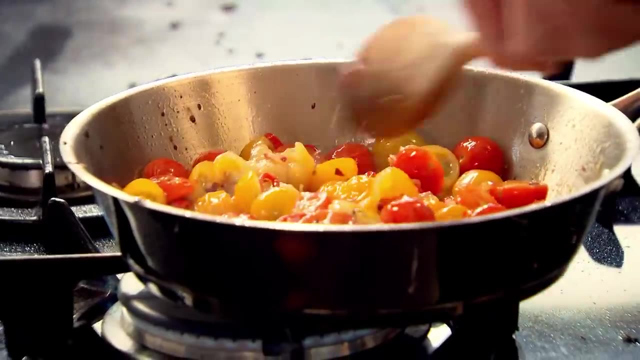 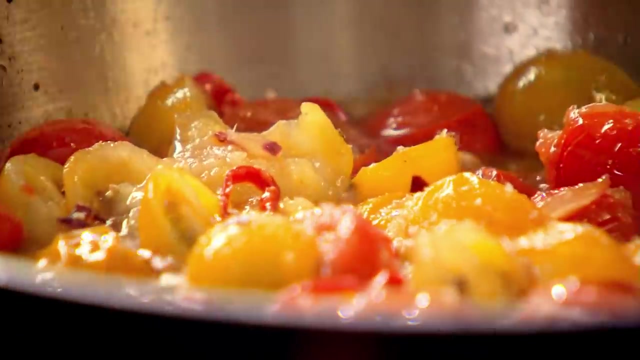 Take a wooden spoon and just sort of break them up. Once the skins blister, the whole tomato just starts to release all that really nice sweet texture. A little teaspoon of sherry vinegar gives that nice acidic balance. the sweetness of the tomatoes. Turn down the gas and just let them sort of cook. 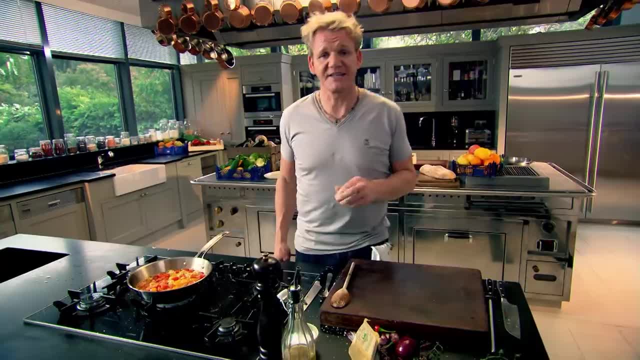 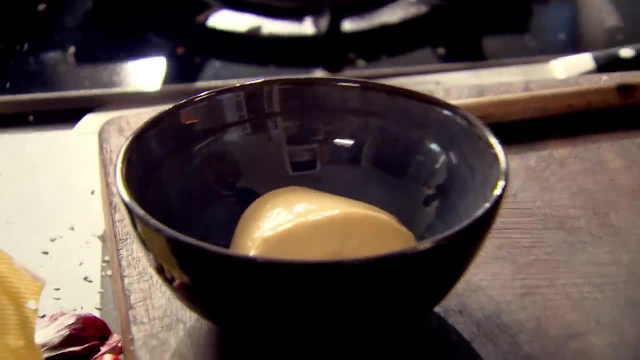 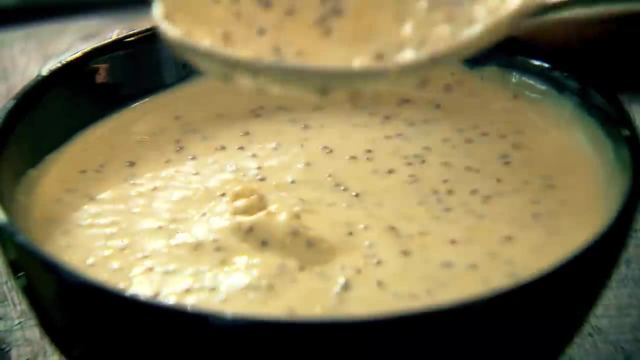 It's going to give it a nice little bit of stew, perfectly. Now, a steak sandwich would not be complete unless it had the most amazing mustard: mayonnaise. Simply add three tablespoons of mayonnaise to three teaspoons of whole grain mustard. Now I've got the relish almost down to like a really nice jam. 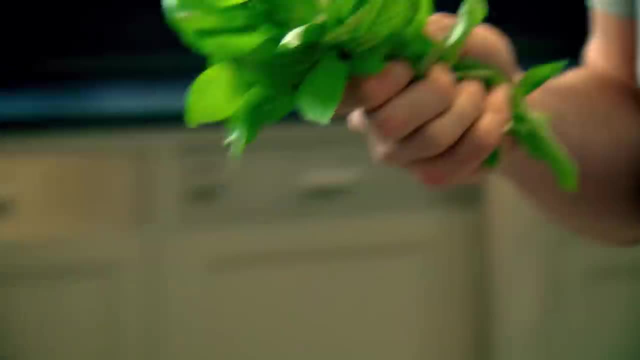 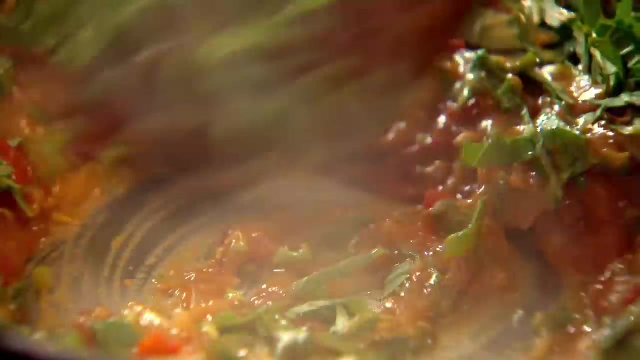 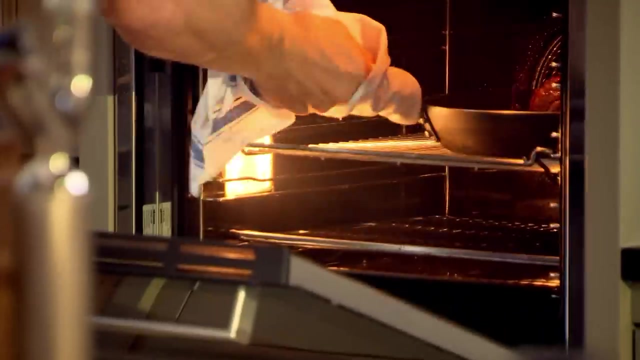 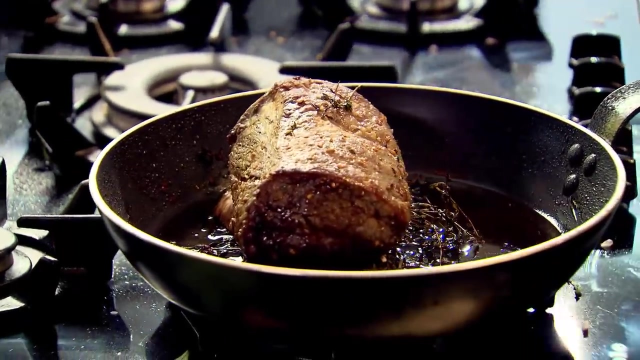 Now I want to make that relish a little bit more fragrant. Some basil, Slice it through. Sprinkle that basil in there. Mmm, Beautiful, Look at this. There she is, My crown jewels. Time to take it out.